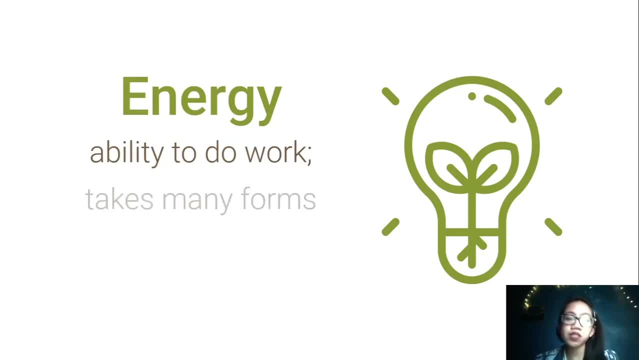 and in our universe it may come in different forms. So first mechanical, then C stands for chemical, T for thermal and then E for electrical energy, And the last one is what we have been using in the past century, So relying highly on electrical energy in our day-to-day activities. 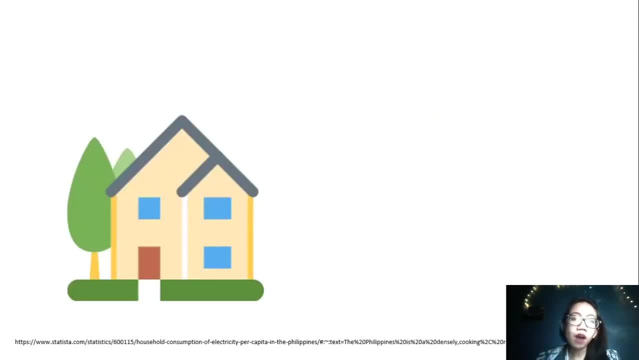 Okay, so, speaking of day-to-day activities, how much do you think electricity does the Philippines actually use? Now, this is a data from 2015.. So the Philippine household consumes an average of 248.1 kilowatt per hour. So, if you are curious, if you are following this average, you could go. 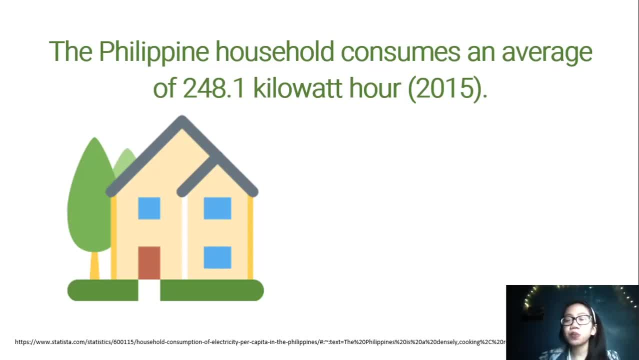 ahead and take a peek at your alcohol bill if you are next to this average. But again, this is an average 248.1 kilowatt per hour. So we use this mainly for lighting purposes, So to power up our light bulbs, our LEDs, Next cooking. So either you have an electric stove, you use it for. 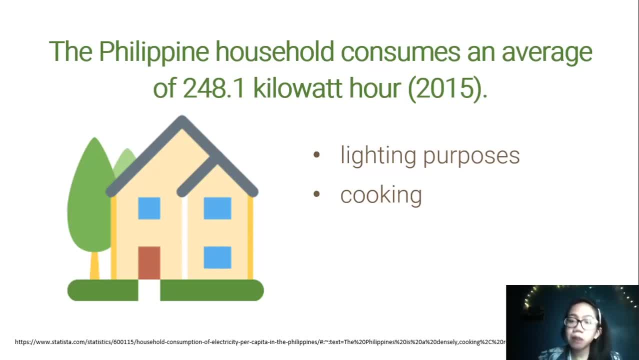 the microwave, your toaster and other kitchen appliances. Next, recreation: So watching TV, home cinema, playing games with your PC- Those are included in the recreation part. Next, space cooling. So, as Filipinos, it's very hot here in our country, So we use a lot of electric. 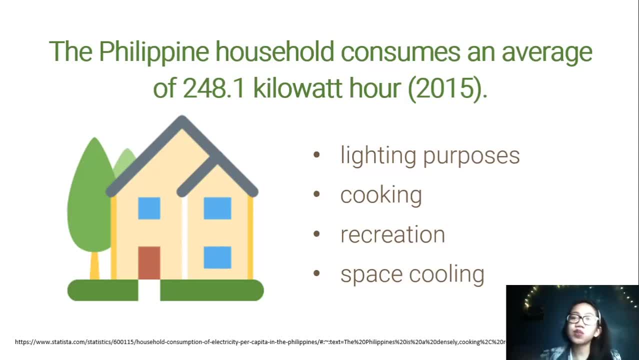 fans and air conditioning. So those are our main uses in terms of electricity. So very simple in terms of the Philippine perspective. So 248.1 kilowatt per hour is what the Philippines uses. This is our average for the Philippines, But how about the world if we look at it? 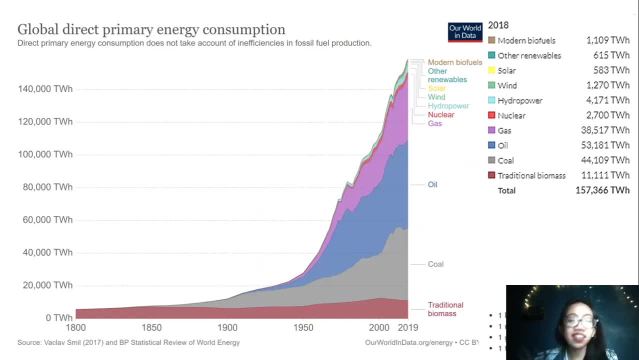 So this amazing graph- I really like this graph because it's giving us a lot of data- is the global direct primary energy consumption as of 2018.. So it's giving us the amount of energy we actually consume per hour. So, according to this 2019, this data- 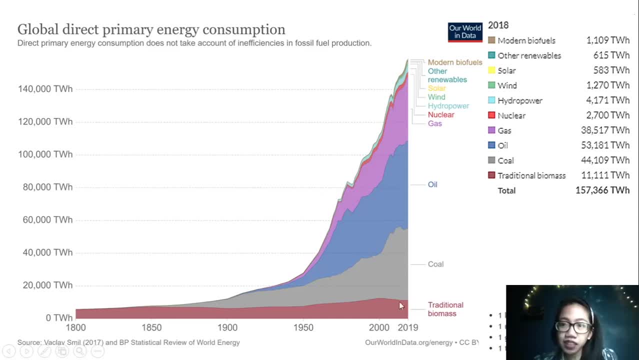 this is projected data because the data came from 2018.. So it means it sort of projects how much we consume by 2019.. Okay, And since we have been increasing in the use, I think it still follows. So, according to this global direct primary energy consumption data table, we have used about 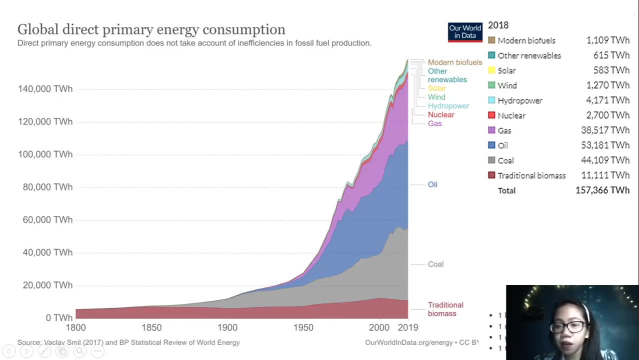 151,000 terawatts per hour. So if you're curious what the H stands for, that's terawatts per hour, as indicated here on the bottom left. Oops, you don't see it because my face is there. But yeah, terawatts per hour it's going to be in. 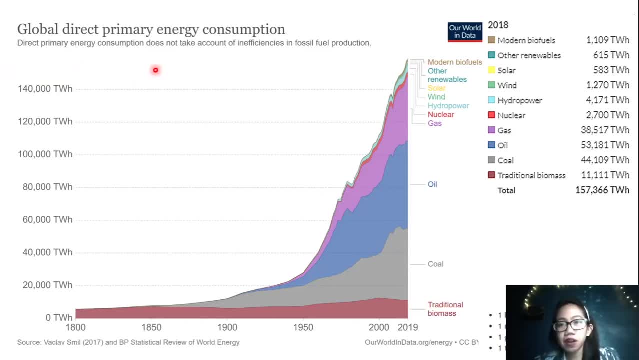 the slides. So 150,000 terawatts per hour by average by 2019.. And as you also see on the right of the table, it's showing where we actually get the energy that we consume. So the lowest one, traditional biomass. So when we say traditional biomass, basically 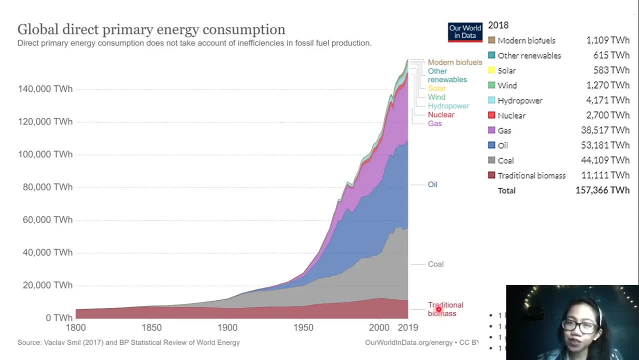 using firewood as a source of energy. Next we have coal, followed by oil and gas. So these three are the big players in our energy consumption, And then the small fraction would have nuclear, hydropower, wind, solar and other renewables. I'll also include the modern biofuels. 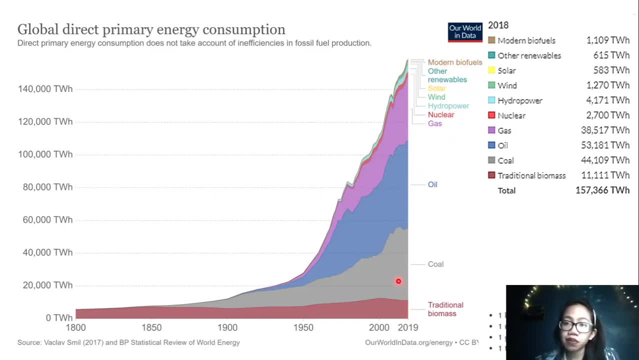 Clinically there is no. digital technology is significant And obviously we don't have any information about the production scheme of oil and gas in fugitive water, But it seems that the world today is still highly dependent on these three: gas, oil and as well as. 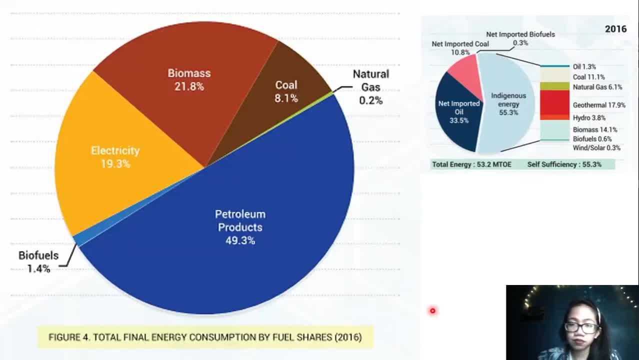 coal. So let's go back to the Philippine perspective. So how does the Philippines generate electricity? Or how does the Philippine? where is the Philly Peace out운? Hello, um, please make sure that you type in the Q&A and I'll be answering any available questions, if you have. so just give me three minutes so I don't need your call out now, right now. Thanks, bye. 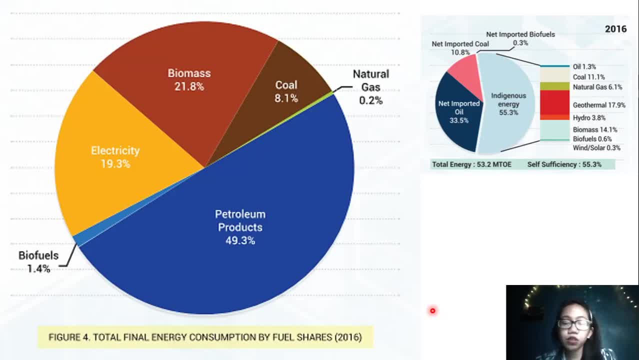 where is the energy of the philippines come from in terms of resources? so, as you can see here, 50, almost 50 percent of our of our energy comes from petroleum products, then 8.1 from coal. we also have biomass sources. so, as i mentioned, um fire, like cooking with firewood or charcoal. that's still. 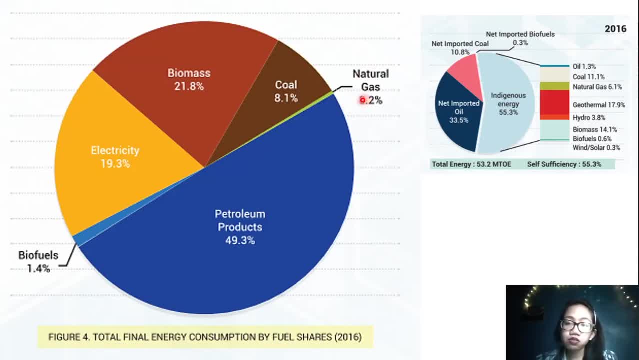 a form of biomass. we have a small percentage- 0.2- of natural gas, and biofuels are of 1.4 percent, now for electricity, 19.3. of course, we have to generate that from other resources, so it could be from fossil fuels or renewable energy. okay, so in terms of the philippines, we are not. 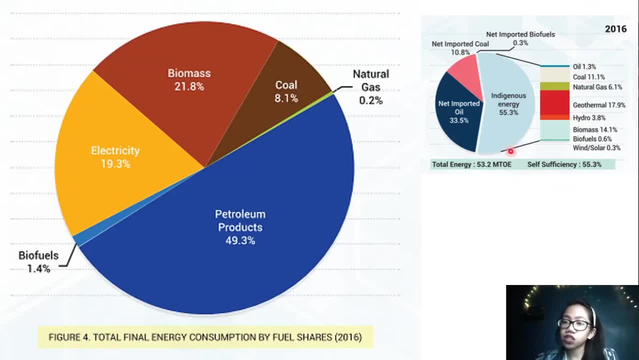 self-sufficient in terms of our energy. we can support ourselves here. in the genus energy is 55.3, so we can produce um or support 50 or 55 percent of our energy demand, but the rest have to be imported from other countries. that's why we have to buy oil either. 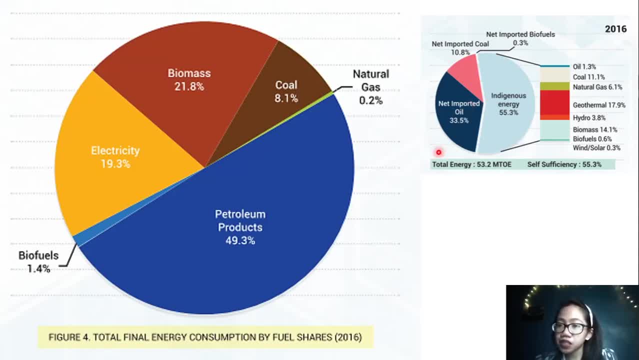 from the united states or from the middle east, okay, so just gonna give you time to like digest this graph, okay, all right. so, uh, this is what we will be discussing one by one. so what are these energy sources that i am showing you, and where do we actually get them? okay, so this is the philippine. 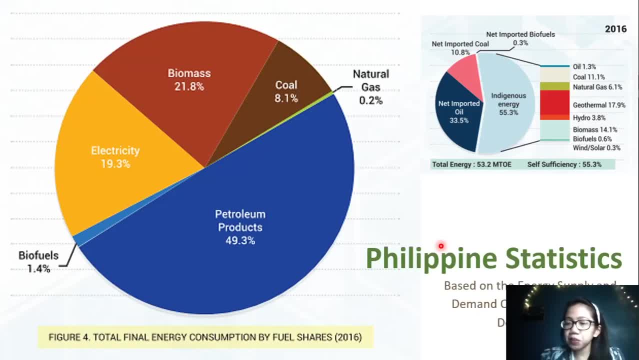 statistics. by the way, this table is from the philippine statistics provided by the department of energy um report in 2019. um, just a quick, like a quick segue. the philippine department of energy has not produced data since 2017 and i don't know why they used to like giving these graphs, these very organized graphs that. 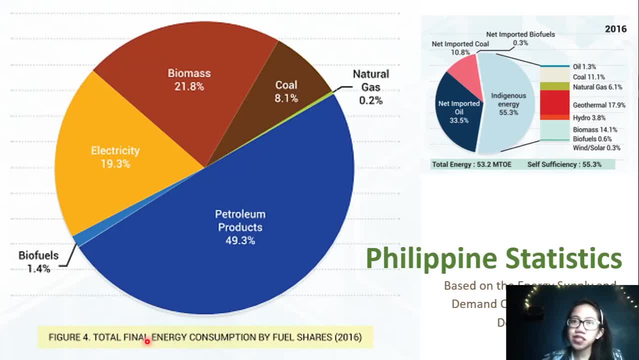 you see on your screen, but since then we don't see a comprehensive review of how much we actually generate versus the demand, and i i have some assumptions, but of course we're not going to discuss that. if we'rekomore correct, discuss that, since this is not politics class. okay, so the energy that i have shown you in the 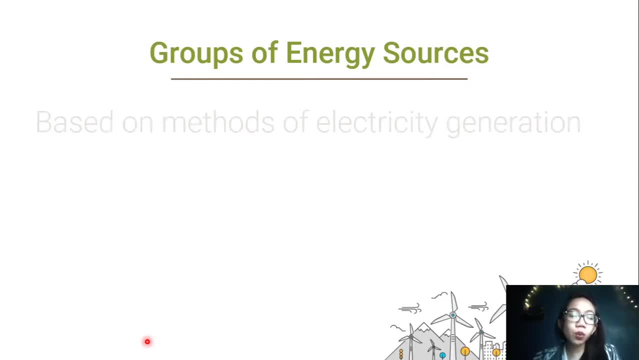 graph can be grouped into different energy sources. so there are two. so, based on the methods of electricity generation, this could be renewable. so those energy that is not reliant on sources that are finite or has a limit, so renewable is from unlimited resources. then when we say non-renewables, those are the conventional and canned and are limited. 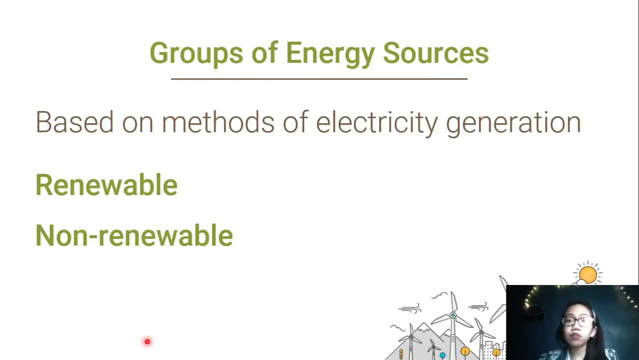 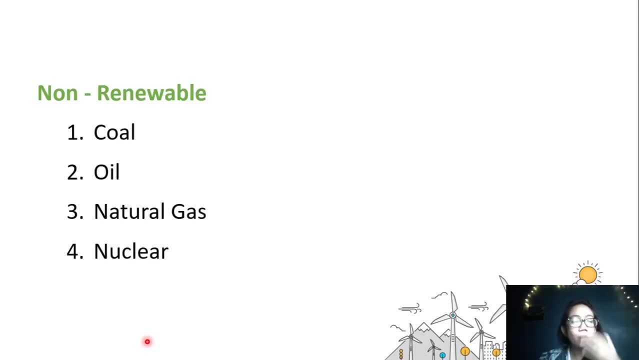 so there is a possibility that we will run out of those resources in the future. okay, so for the non-renewable we have four, so coal, oil, natural gas and nuclear power. then for renewable energy we have quite a few. you have your solar, wind, hydroelectric, geothermal. 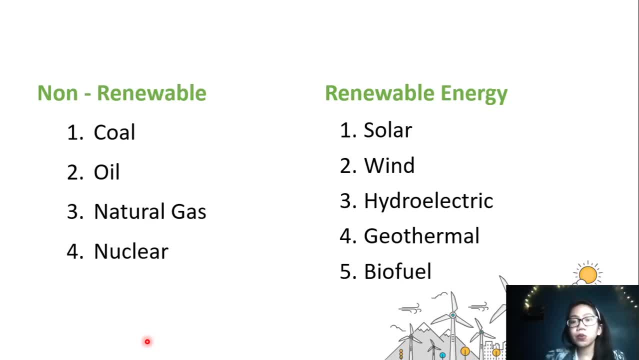 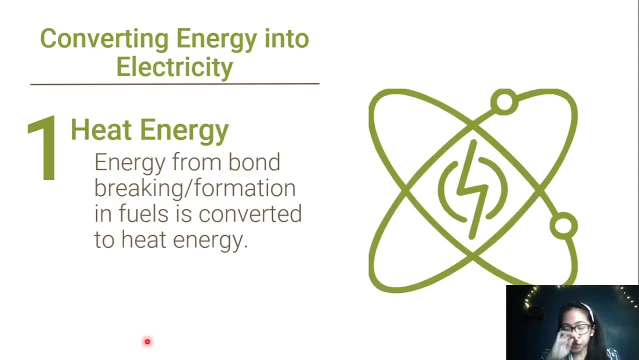 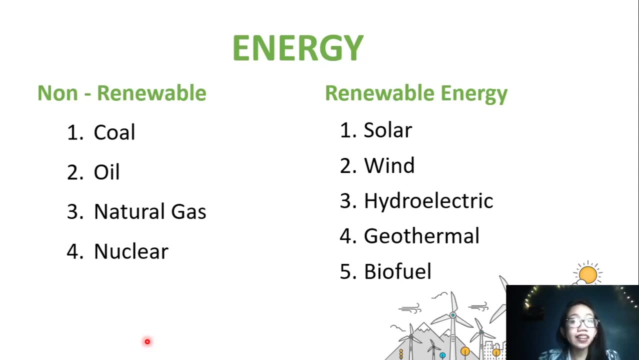 and, of course, biofuel. so we're going to go through all of these types of energy during our module discussions. okay, but before we jump into the main discussion, the, as you can see, there are like nine types of energy listed here, but the way we produce electricity- electricity using all of these resources- are pretty much the same. 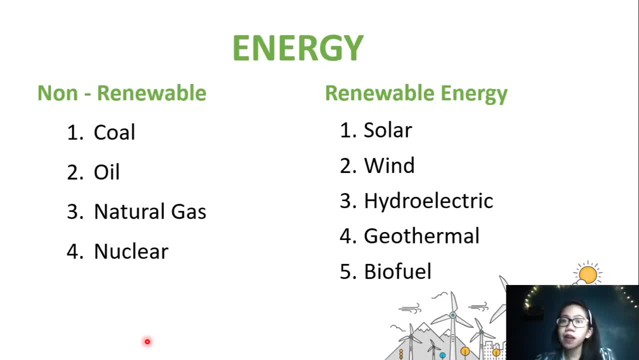 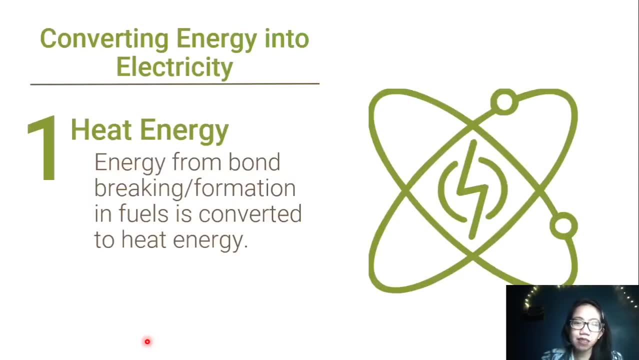 the main idea are the same, step by step, step-by-step. the end goal is electricity And if you summarize it, they do have their own same mechanisms. So first we rely on heat energy. So whenever we want to convert the energy that I 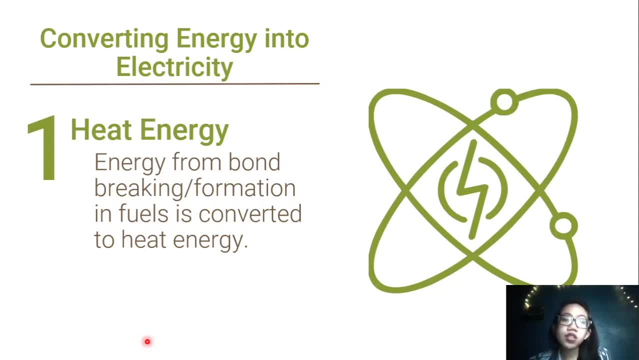 have shown you energy resources that I have shown you. it usually starts with heat energy, especially the fossil fuels. So energy, heat energy, energy from bond-breaking formation in fuels is converted to heat energy. So, for example, if it's a fossil fuel, we use it to combust something. 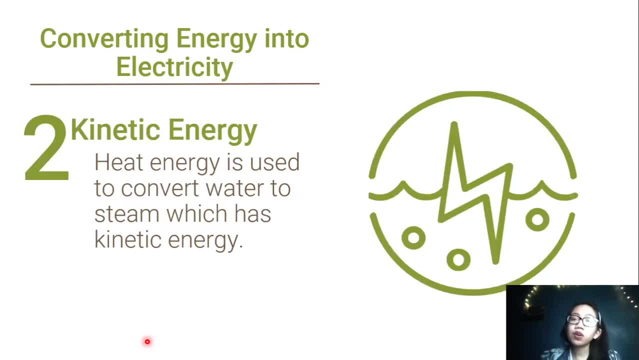 in order to create heat. Now that you have heat, we will convert that into kinetic energy. So the kinetic energy is from the heat energy used to convert water to steam, which has kinetic energy. So basically, using your heat energy in order to boil water and in that you have